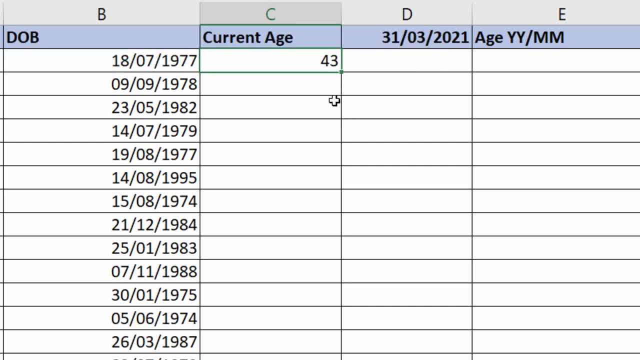 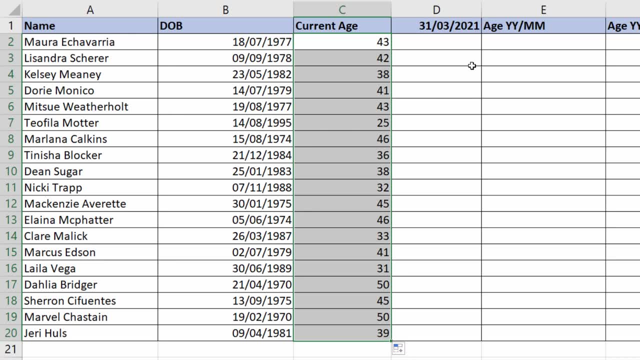 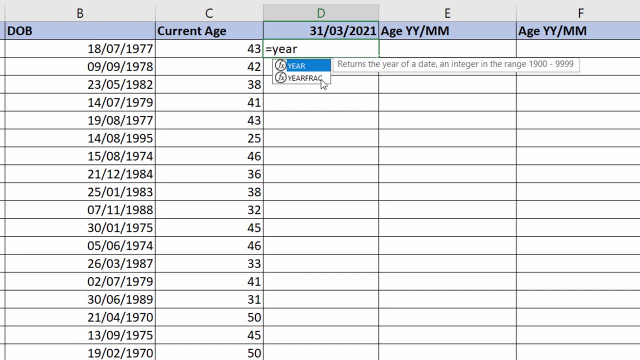 the integer of that calculation, Put it down. and there we are. I have the current age for each of our members of staff. If I want to calculate their age on a specific date, say in the future, same thing, really Use yearfrac. Start date would be their date of birth. 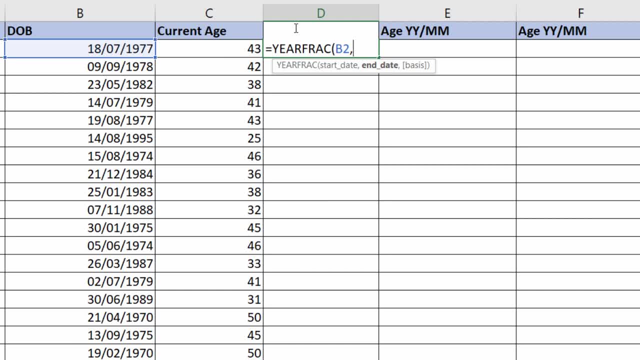 Comma. end date would be D1, where you've got the date, I can't click into it, so I'm going to type it in. You need to fix it because you're going to be copying this down. I used F4 to fix it. If F4 doesn't work, then type the dollars in. There's one before the letter, one before the number. 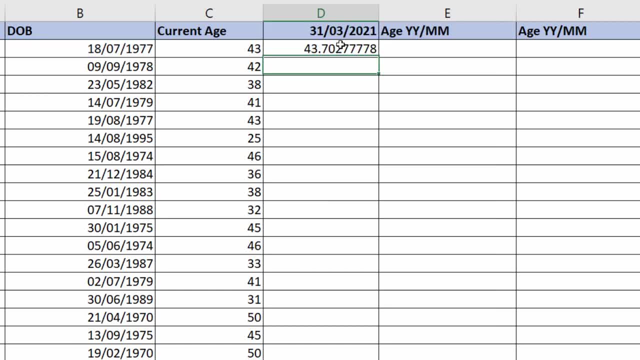 And again to return an integer, use the integer function, Copy it down and you have their age on a specific date. To show the year and month portion of their age a little bit more involved, we'd use a function called DateDiff. It won't appear in the IntelliSense list. DateDiff has three arguments Not shown in the screen tip, unfortunately. 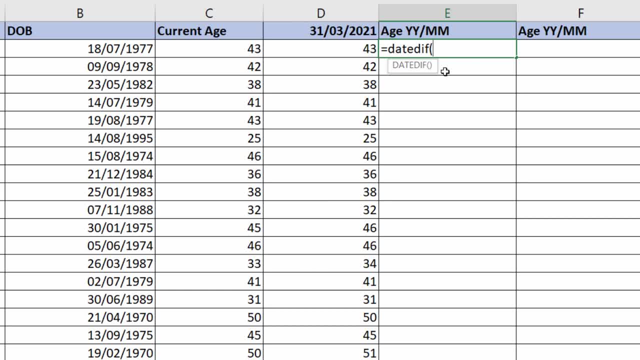 DateDiff has three arguments not shown in the screen tip, unfortunately: Start date, end date and then the unit of the calculation you want to return. If you want to return the year part of their age or the month part of their age, You can only return. 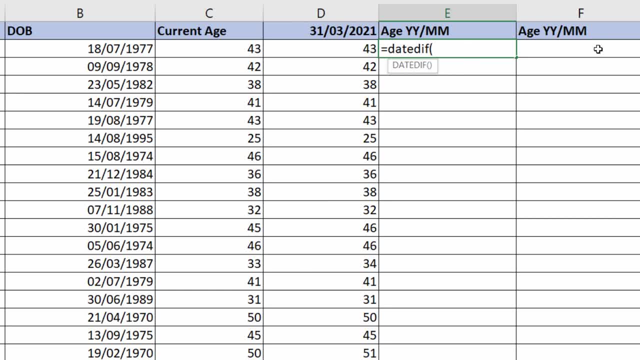 one unit at a time. so we're going to have to do two DateDiff formulas and then concatenate or join them together. We'll start off with year. Start date would be their date of birth, End date is today's date. Then we want to calculate the year. 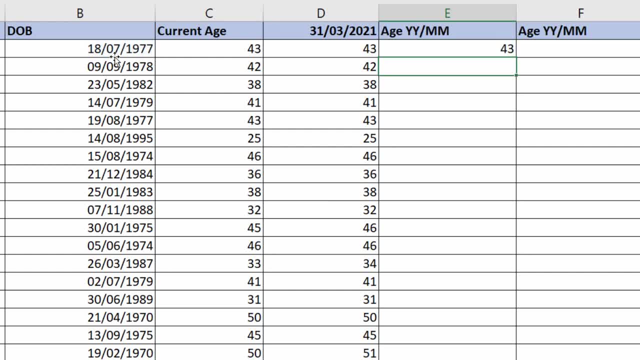 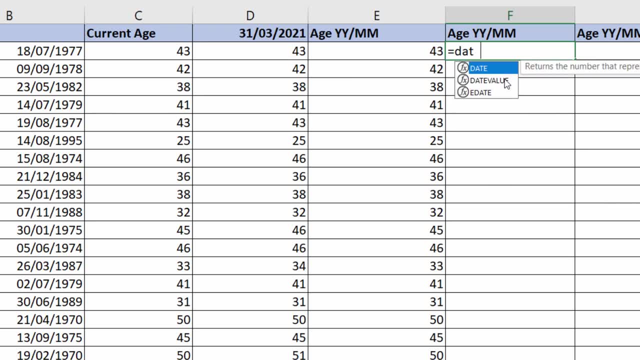 In quotation marks. you put your y in close the bracket and it returns the year part of their age For month: DateDiff: Same thing, their start date, the end date, today's date. Now, if I put in m, you'll see that what it does is return the total number of months, not the number of months over. 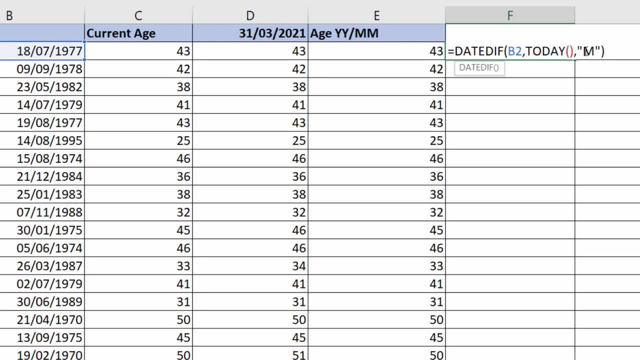 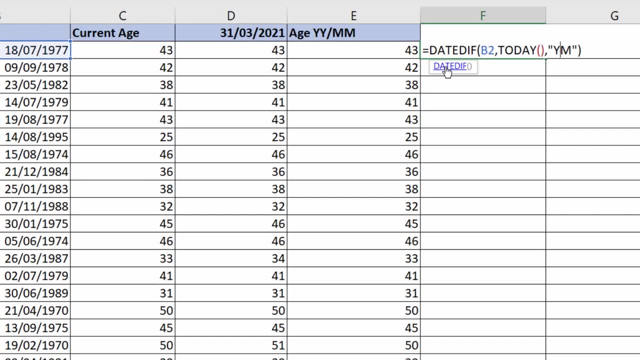 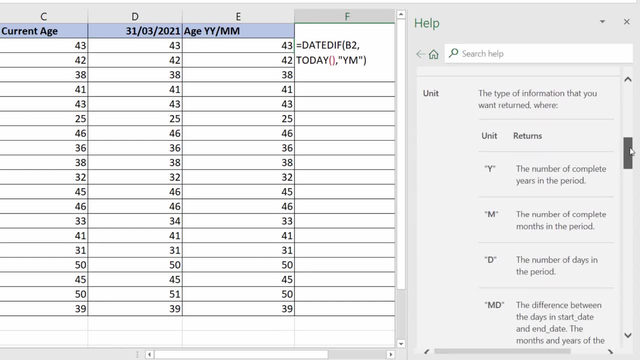 their age in years. So, as you can see in the screen tip, the y is the end date. To get around that, all you do is you put y in front of that m. Now to understand that if you click on this little link here in the screen tip, it'll either open up a